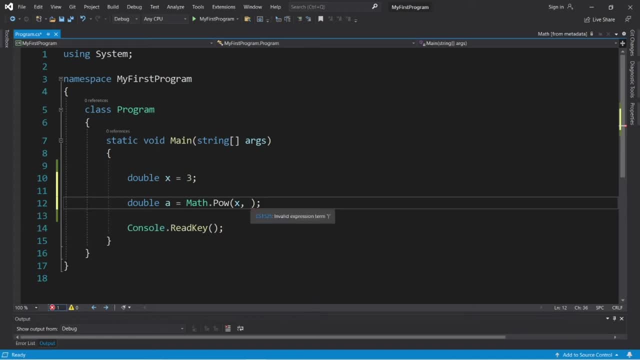 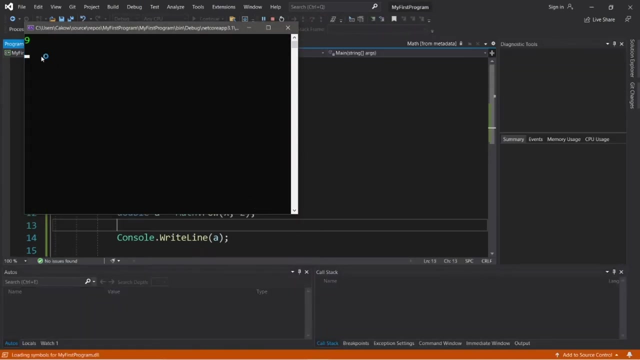 And what power do we want to raise x to? Let's raise x to the second power and then display, whatever our result is, a. So, within a right line statement, I'm going to display a. So here is the result: 3 to the power of 2 is drum roll, please, 9.. So if we need 3 to the power of 3,, 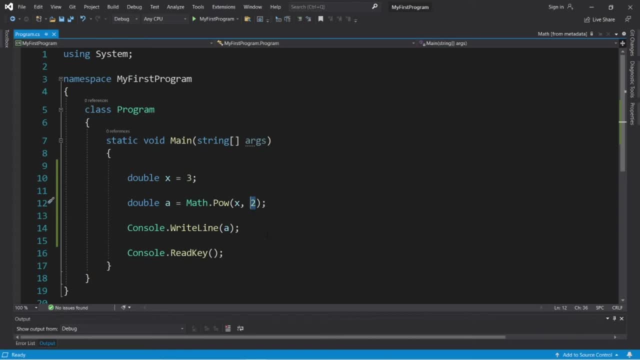 that would be, you know, x. whatever you're working with, that's the base comma 3.. So 3 to the power of 3 is 27.. Okay, let's try square root. I'll turn this line into a comment and we'll. 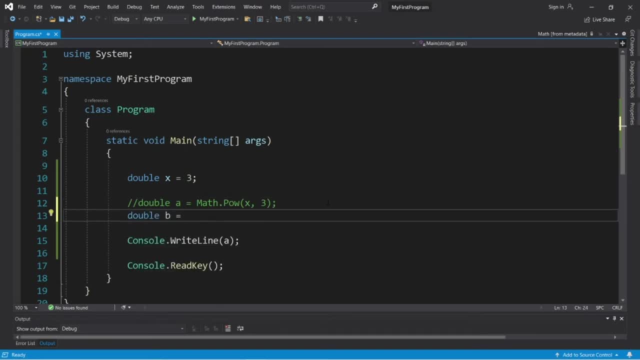 create double Double. b equals then again to access methods from the math class type math with a capital, m, dot, and we are looking for square root. That is all the way down here: sqrt- parentheses, semicolon. within the parentheses we will find the square root of x and then store it within b. 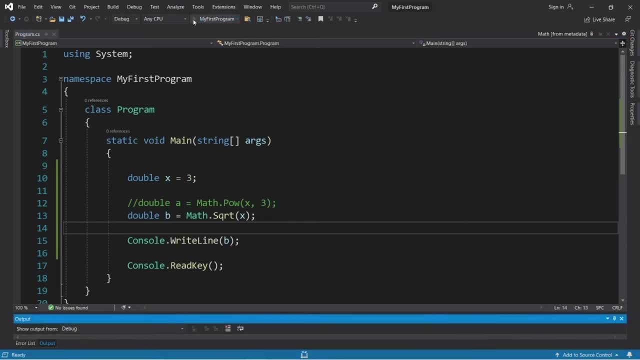 Console. dot right line b, And that would be 1.. 7,, 3,, something, something, something, something. So that is the square root method. Let's move on. Let's create double c and we'll find the absolute value of x. So math: dot a, b, s. 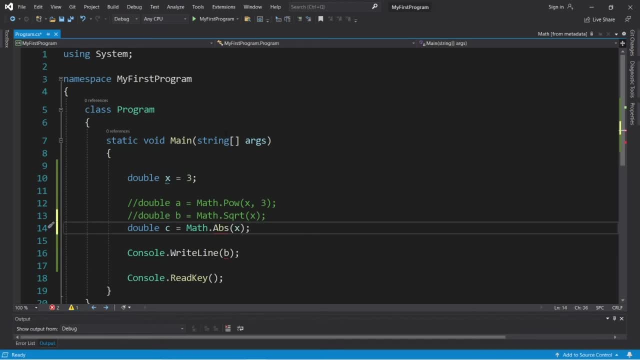 So the absolute value is how far away something is from 0. So if you have a negative number, like negative 3, well, it's going to turn that into a positive number. So the absolute value of negative 3.. We need to display c. 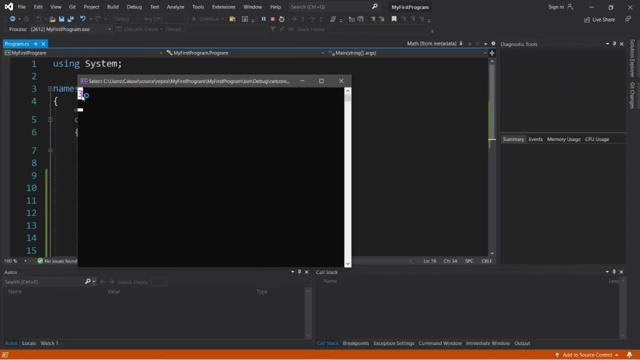 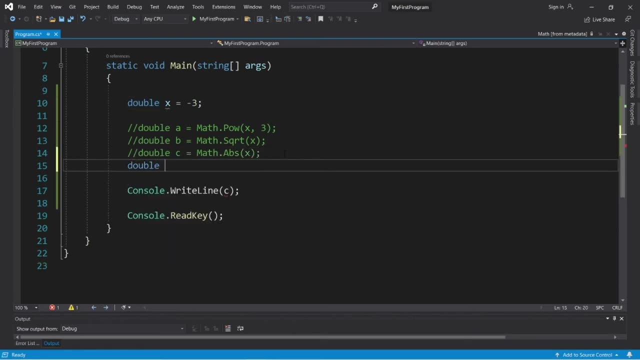 So the absolute value of negative 3 is in fact 3.. So that is the absolute value method. Let's move on Rounding, So double. let's see we're on d equals math, dot round and we can round a number. Pay attention to the capitalization too. 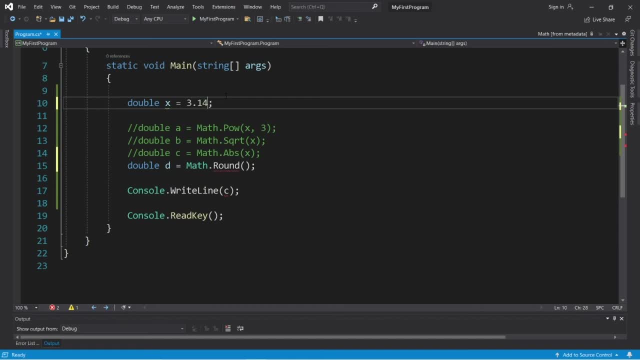 Okay, now let's change x to 3.14, and then we will round x. So place that within the parentheses of the round method And we will display d And 3.14 rounded is 3.. Now you can always round a number up by using the ceiling method.